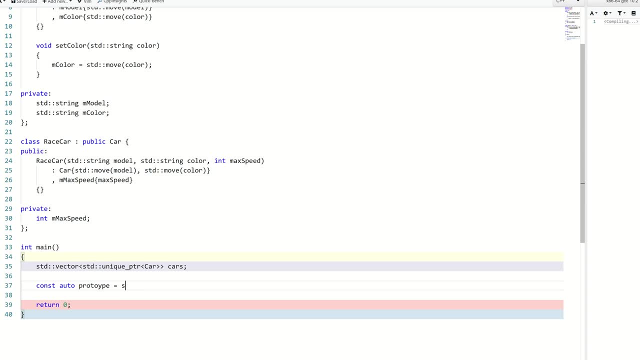 auto prototype type will be make uni over race car. We will call it, for example, awesome car with an empty color for now and some max speed. Now we need a way to clone this prototype, So let's add a clone method in our base car class. of course, We add: 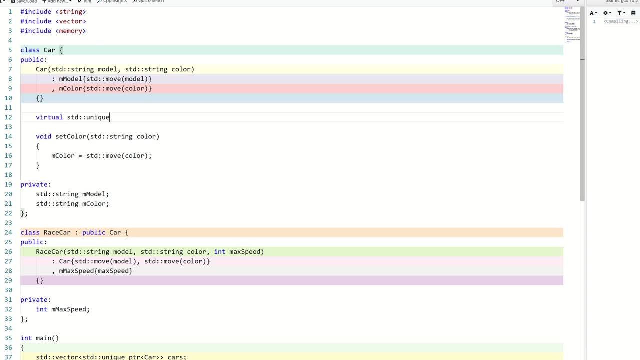 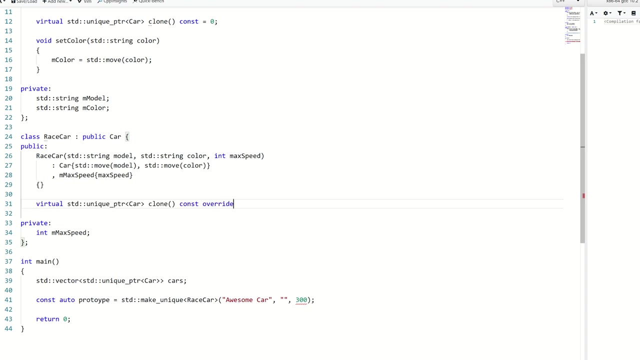 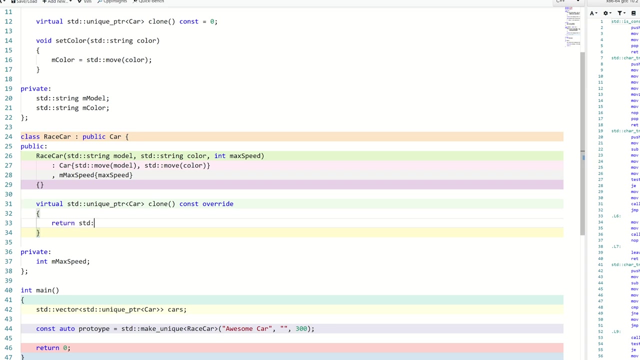 virtual std uni pointer of a car. it's called clone, And let's add our implementation to a race car. We will simply leverage the copy constructor. so return std, make uni over race car inside. simply pass this then, instead of making new awesome cars which only differ in. 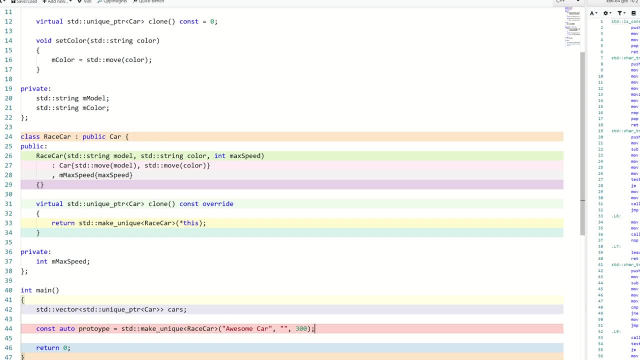 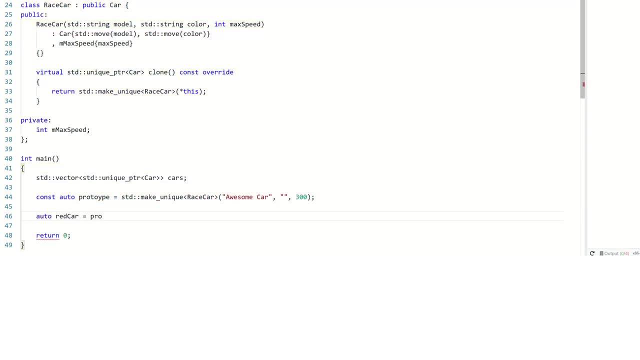 color. we can simply clone the prototype and set the color to whatever you want. for example, if you want a red car, we can write: red car is simply proto type clone and let's set its color to red. ah, a typo. we now have a red car and we can add it to our inventory. so cars. 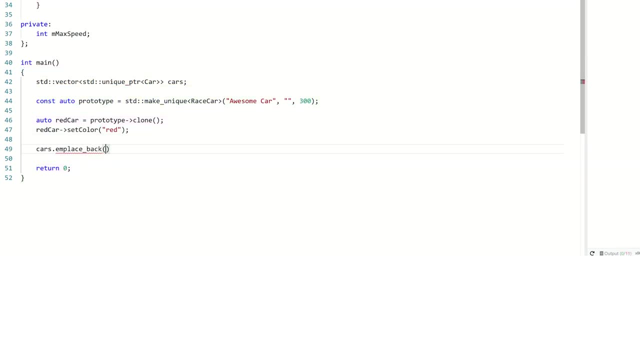 and place back std, move red car and that's pretty much it. if we wanted another car, for example a blue one, you can simply copy and paste that but switch red to red, blue, blue here, blue here and blue here, and now we have both a red and a blue car without any need. 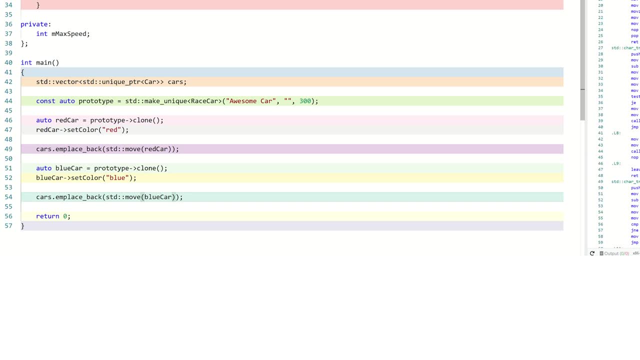 for builders or abstract factories. so what are the advantages of this pattern? we avoid creating additional class keyarchies for set factories or builders. as you can see, we have none. we also avoid repetition for objects which contain mostly the same data. again, the model is the same.